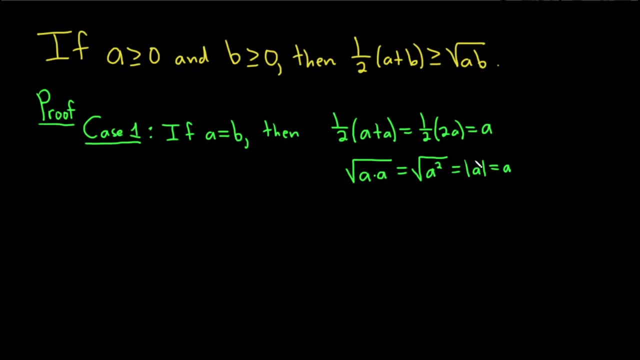 just a. So in this case the statement holds right, Because we end up with a equal to a, So we have a greater than or equal to zero. A is equal to a, which is certainly true because it's equal to a, So that takes care of that. 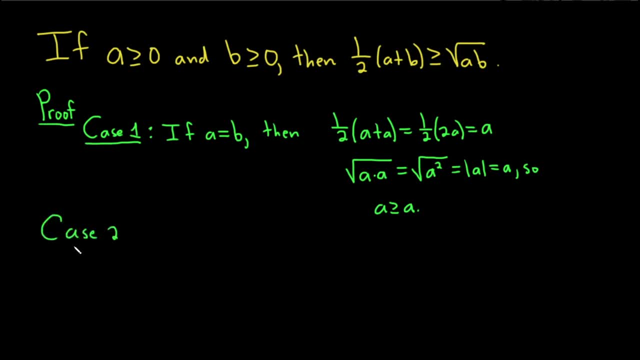 case. Case two would be if a is equal to zero or b is equal to zero. So let's just focus on the case if a is zero. So if a is zero, then we have one half zero plus b, which is one half b. So that would be the left-hand side And the right-hand. 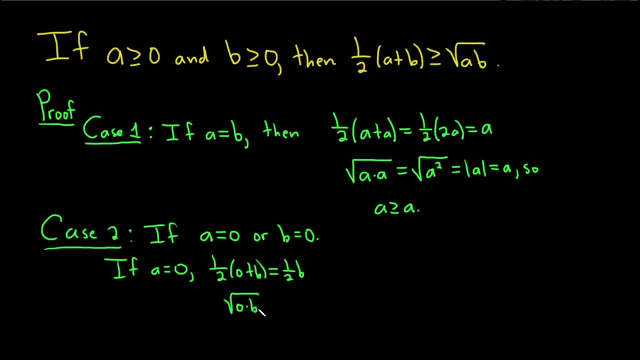 side would just be the square root of zero times b, which is the square root of zero, which is zero. So clearly, one half b is greater than or equal to zero, because b is greater than or equal to zero. If b is equal to zero, it's the same. So, similarly, 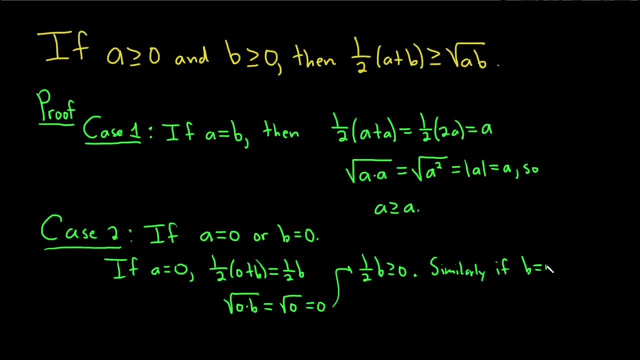 if b is equal to zero, we would have one half a plus zero, which is equal to one half a, which is certainly greater than or equal to the square root of a times zero, which there's your b. Your b is zero because this whole thing is zero, So that's no problem there. 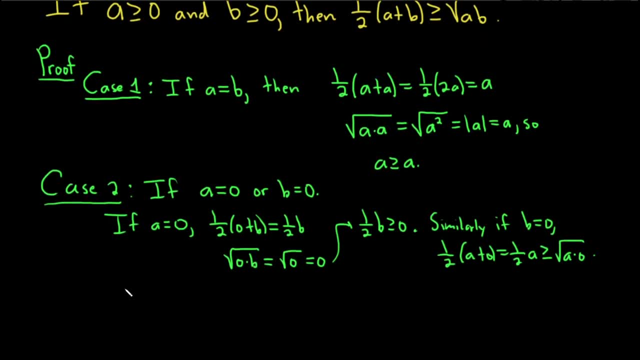 And if they're both zero, both sides are zero. So zero is greater than or equal to zero. So if a equals zero And b equals zero, Then we end up with zero greater than or equal to zero. So everything looks good. So really really easy cases here. Both of these cases are pretty clear. You. 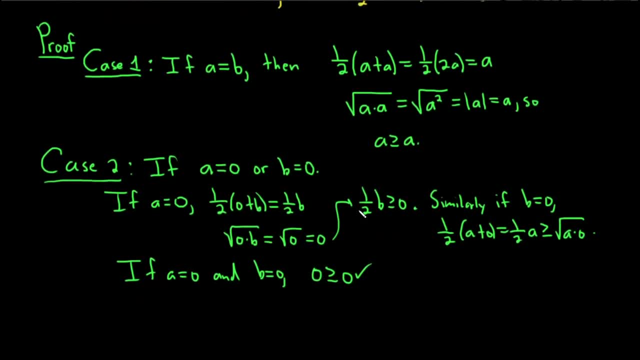 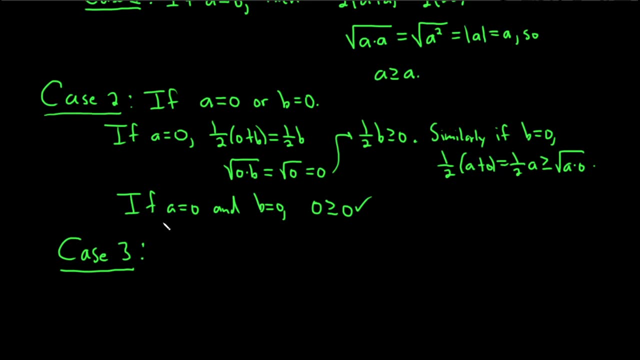 can almost get away with not even having to just justify them. They're very, very clear. Case three will be the hard case. So case three, But you know it's worth mentioning them. So you should at least mention these cases. So totally worth mentioning. So the 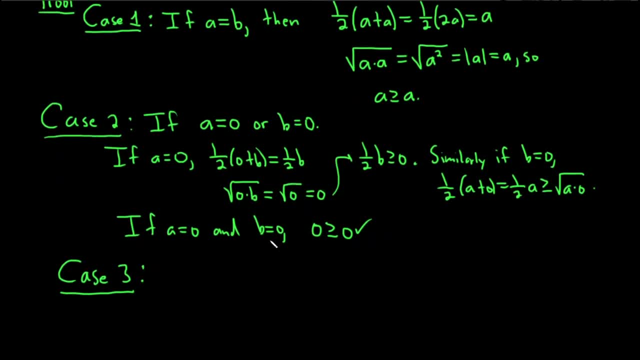 other case that's left is if they're different. So the last case is if a is not equal to b and a is not equal to zero and b is not equal to zero. In this case they're both positive right Because by assumption they're greater. 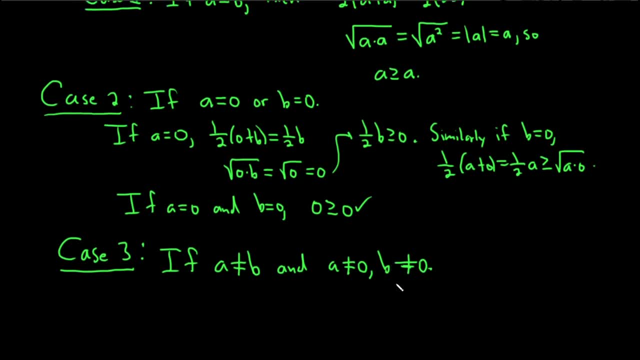 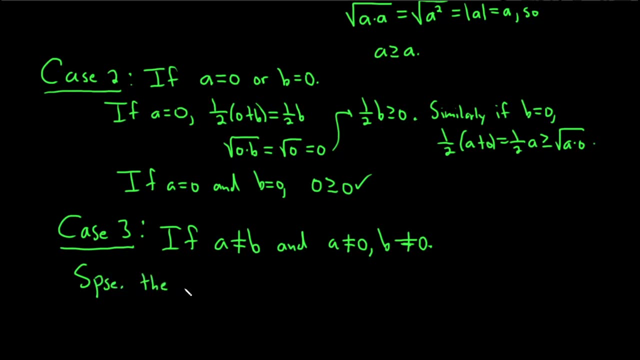 than or equal to zero. So if they're not zero, they're positive. So let's suppose the result is false. So suppose let's proceed by contradiction. So suppose the result is false. The result is false. Hence, well, hence, what do we have? We have 1, half a plus b is less. 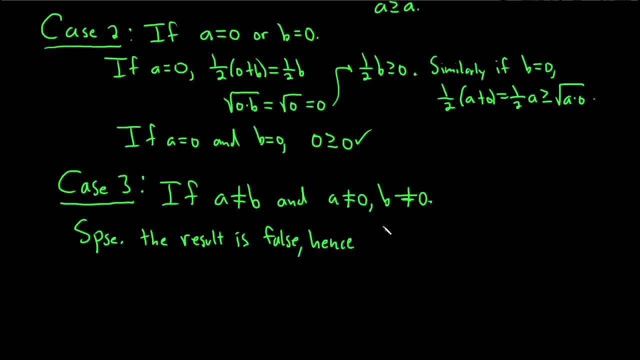 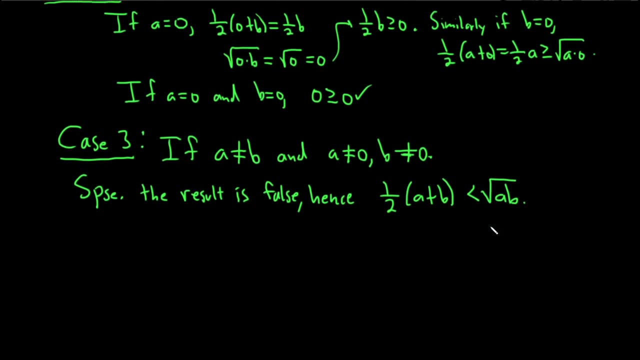 than the square root of a- b. So we have 1. half a plus b is less than the square root of a- b. Then we can square both sides. So then If we square the left-hand side we would get 1 fourth a plus b squared less than square. 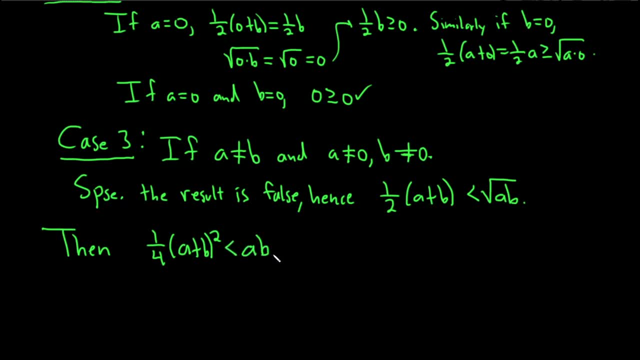 the right-hand side, we just get a- b. Let's multiply this out, So we have 1 fourth. This is a formula. This is a squared plus 2, a, b plus b squared. We square the first one, multiply the a and the b and double it and then square the last, Or you can write it twice in FOIL. 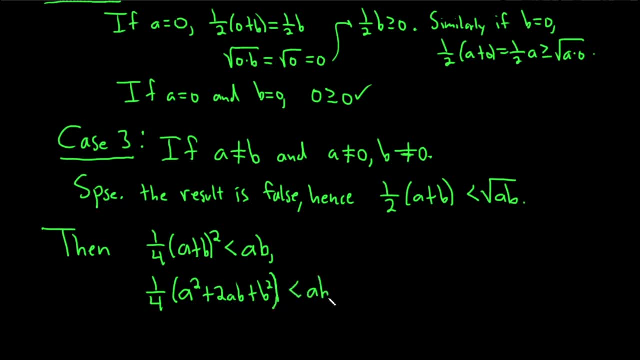 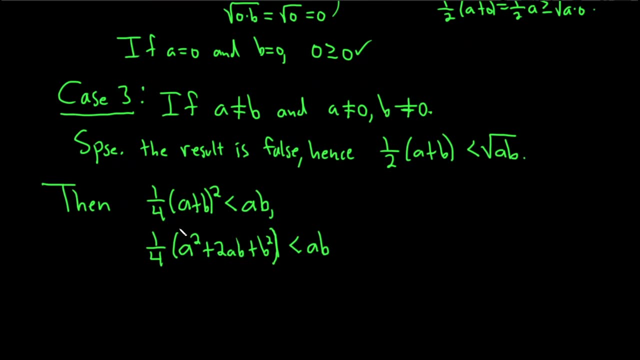 but it's a familiar formula And this is less than a- b And this 4 is kind of in the way. Let's go ahead and maybe multiply by the 4.. So we have a squared plus 2, a b plus b squared, And that's less than 4 a- b. 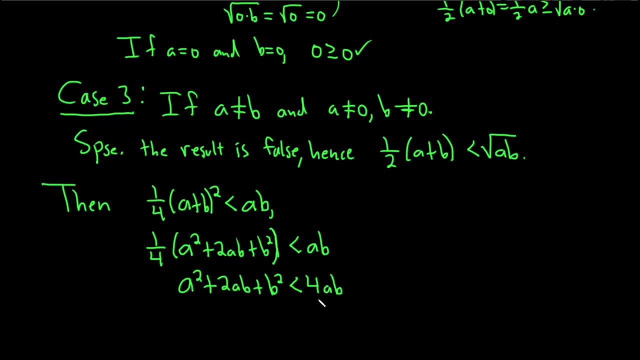 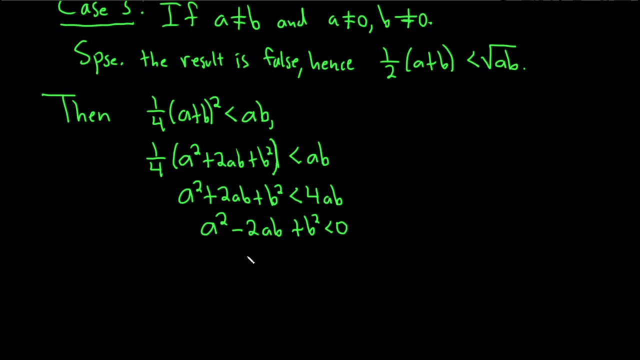 Then we can subtract 4 a- b from both sides. That would give us a squared minus 2, a b plus squared less than zero, And this actually factors. this is called a perfect square trinomial. This is actually a minus b squared less than zero, which is a contradiction, right? 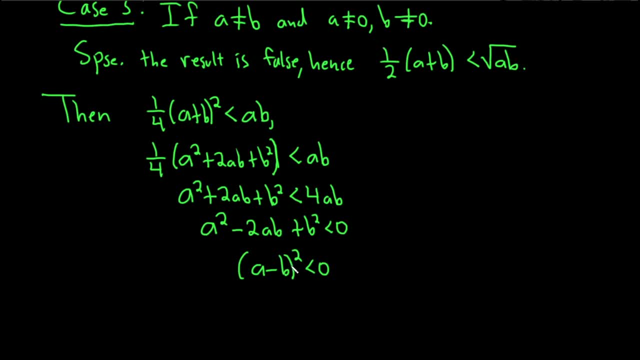 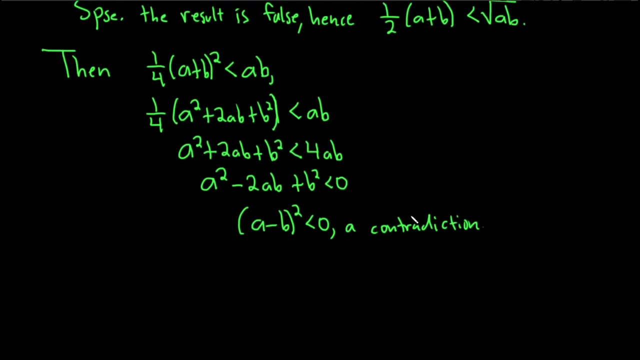 Because this is being squared, so it can't be less than zero, right? It's impossible. So a contradiction, So the result must hold in the last and final case. So we've verified all the cases. therefore we are done, So thus the proof is complete. Thus the proof is complete.